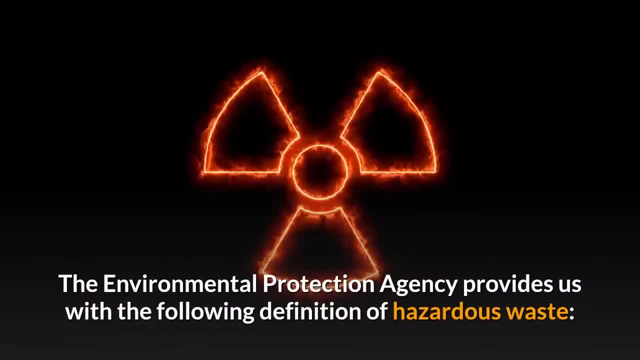 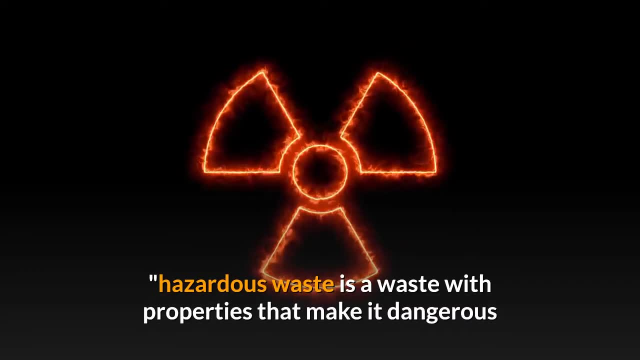 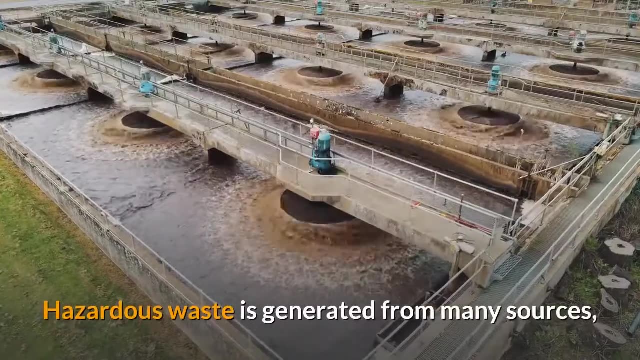 tremendous risks to workers and the public. The Environmental Protection Agency provides us with the following definition of hazardous waste. Hazardous waste is a waste with properties that make it dangerous or capable of having a harmful effect on human health or the environment. Hazardous waste is generated from many sources. 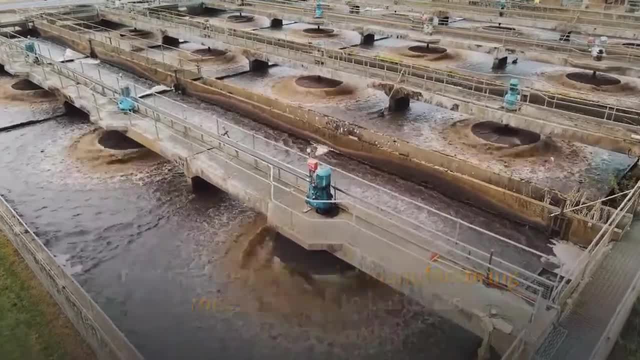 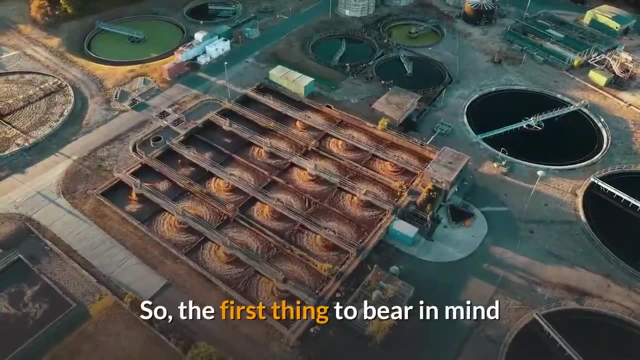 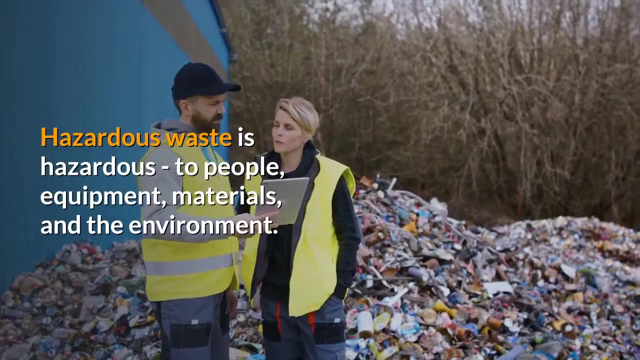 ranging from industrial manufacturing process wastes to batteries, and may come in many forms, including liquids, solids, gases and sludges. So the first thing to bear in mind when dealing with hazardous waste is simply what we learn from its name. Hazardous waste is hazardous to people, equipment, materials and the environment. Treat it as such. 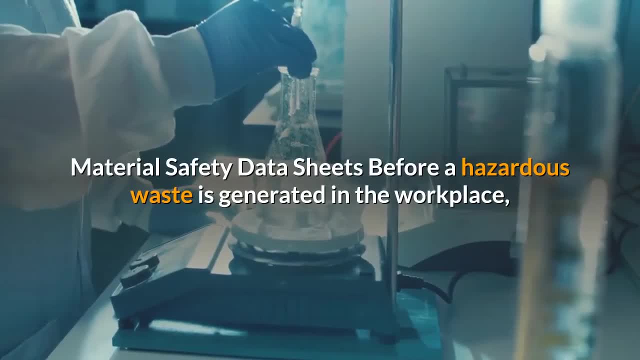 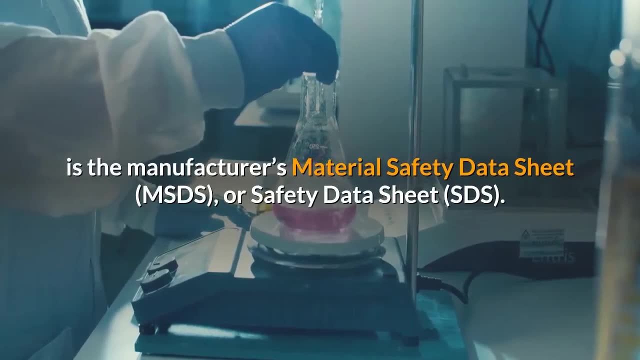 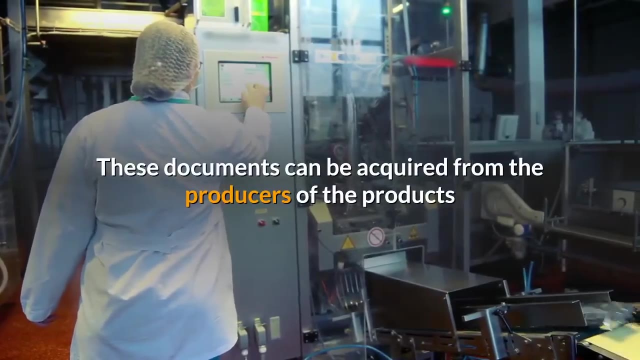 Material safety data sheets. Before a hazardous waste is generated in the workplace, the best place to gather information about its disposal is the manufacturer's material safety data sheet, or safety data sheet. These documents can be acquired from the producers of the products and contain crucial information about the substances. 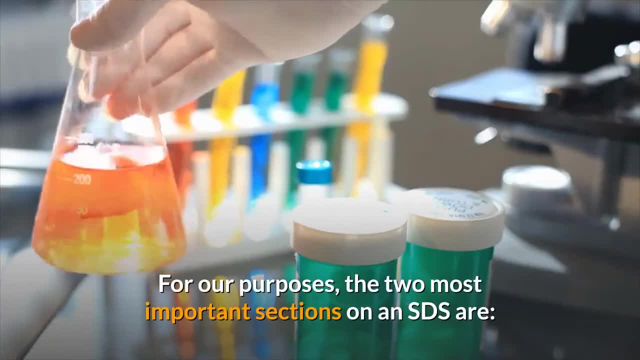 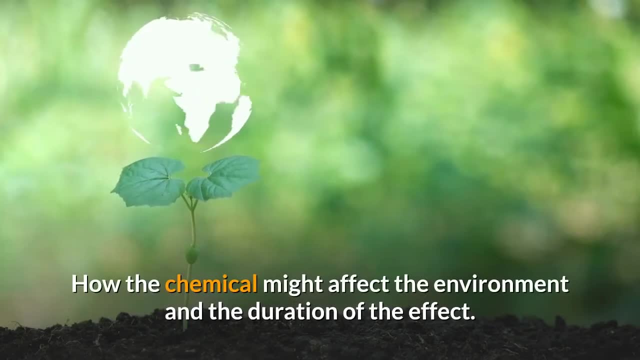 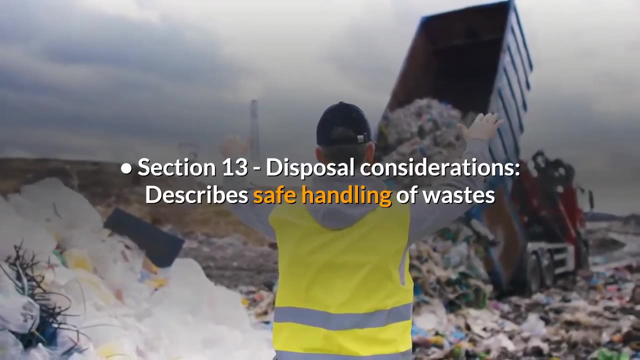 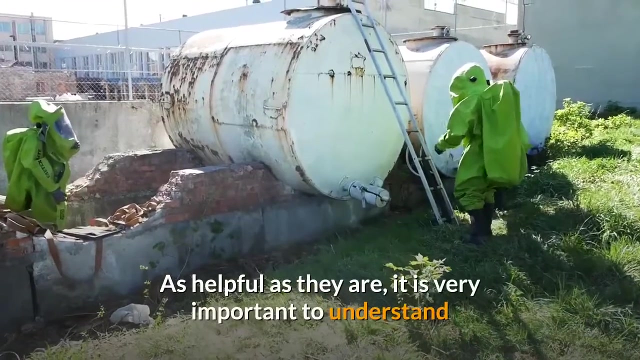 they detail. For our purposes, the two most important sections on an SDS are: section 12: ecological information: how the chemical might affect the environment and the duration of the effect. Section 13, disposal considerations, describes safe handling of wastes and methods of disposal, including the disposal of any contaminated packaging. As helpful as they are, 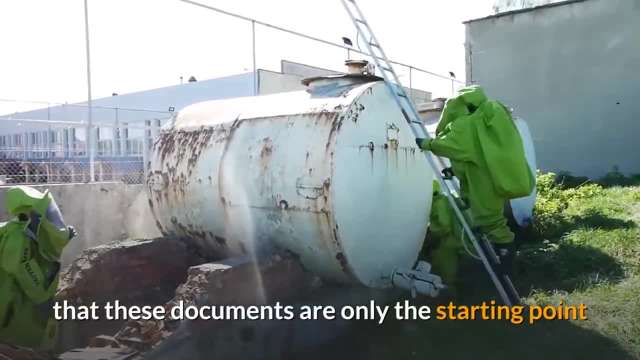 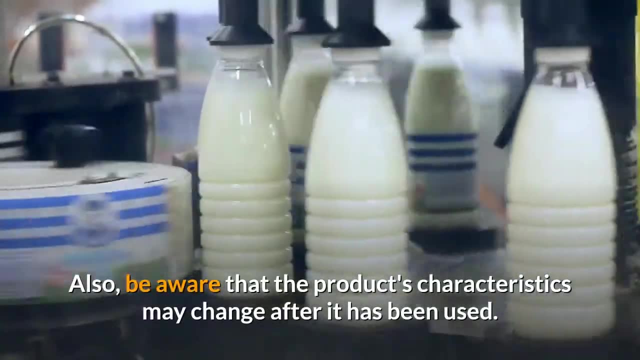 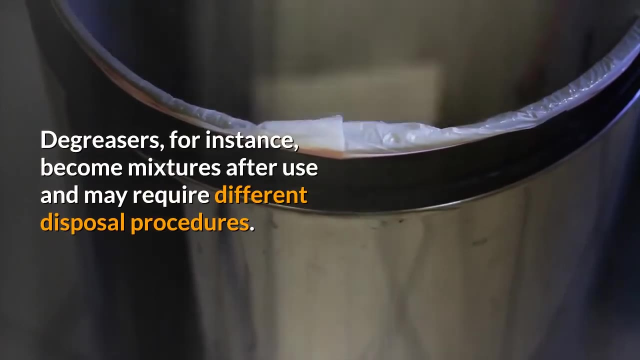 it is very important to understand that these documents are only the starting point for our understanding how to dispose of hazardous waste. Also be aware that the product's characteristics may change after it has been used. Degreasers, for instance, become mixtures after use and may 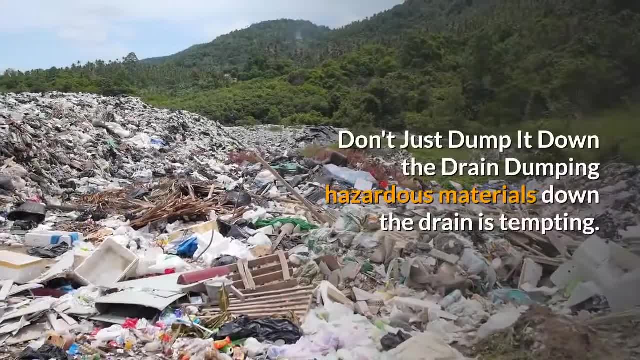 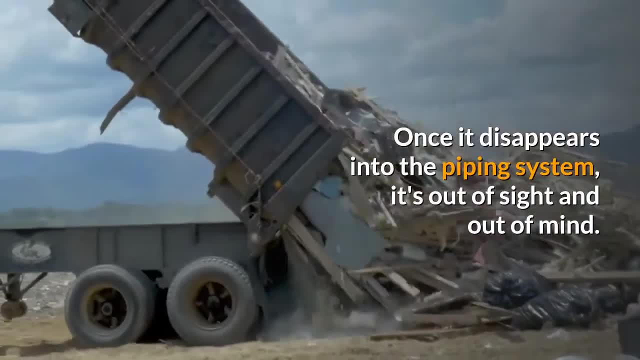 require different disposal procedures. Don't just dump it down the drain. Dumping hazardous materials down the drain is tempting. Once it disappears into the piping system, it's out of sight and out of mind. But that doesn't mean it's without consequences. Section 14: safety data sheets. If the waste is not disposed of, according to the claims of the company, after the waste has been disposed of, it may beевид as the waste is disposed of without clogging the water. DMPD or incineration of the waste In order to minimize the damage caused by the waste. 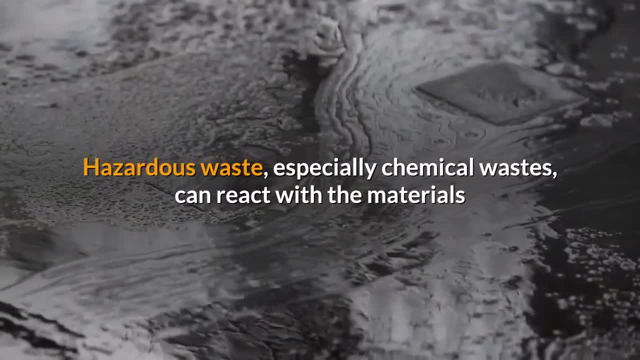 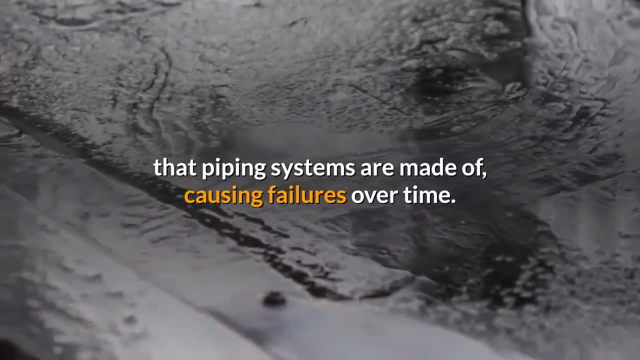 these are the characteristics of the waste. In addition to this, it may also be used as a detergent. In fact, it might even be deadly. Hazardous waste, especially chemical wastes, can react with the materials that piping systems are made of, causing failures over time. 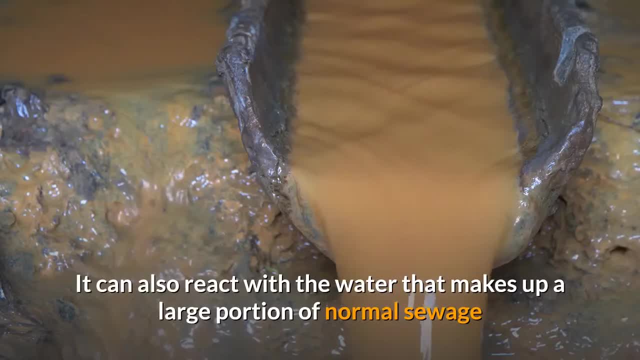 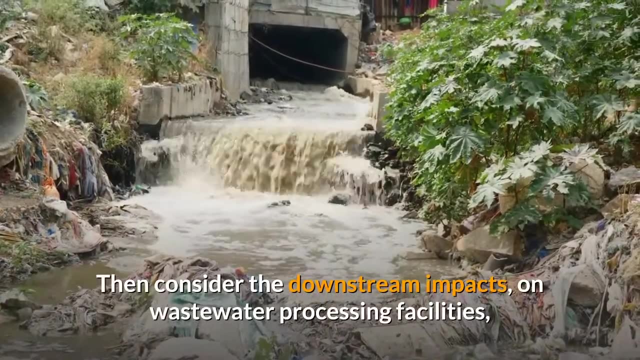 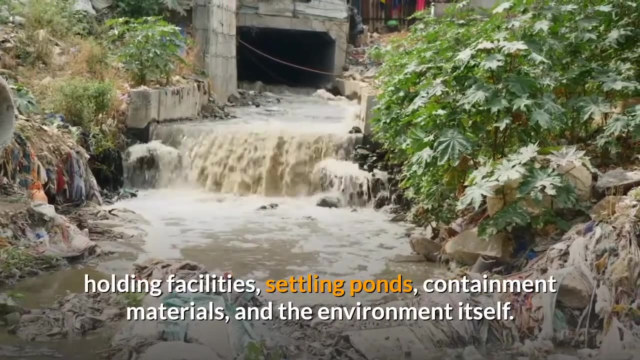 It can also react with the water that makes up a large portion of normal sewage, or with the myriad variety of the contents of the sewage. Then consider the downstream impacts on wastewater processing facilities, holding facilities, settling ponds, containment materials and the environment itself. 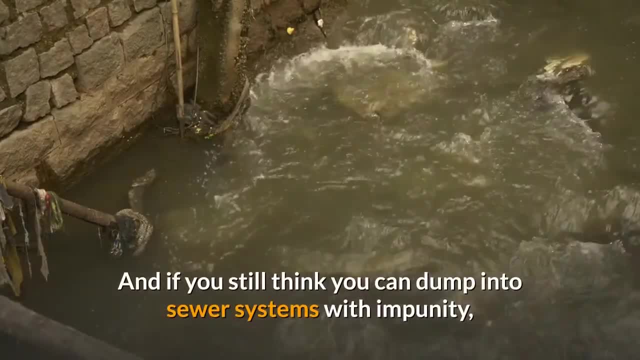 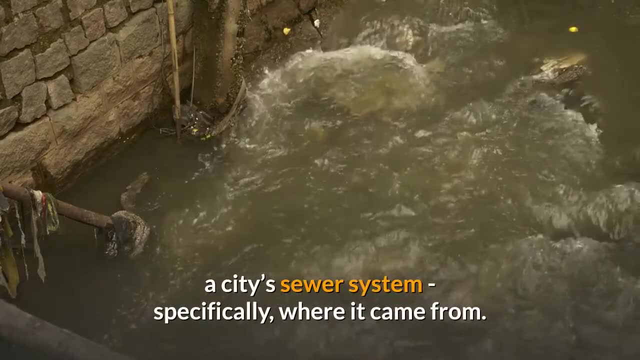 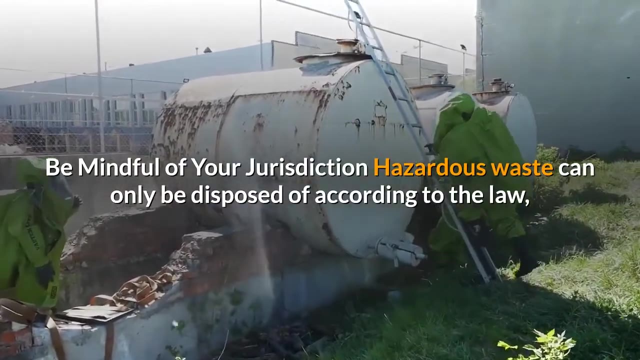 And if you still think you can dump into sewer systems with impunity, be aware that the technology exists and is in common use for tracking in, for example, a city's sewer system specifically where it came from. Be mindful of your jurisdiction. Hazardous waste can only be disposed of according to the law, and there are significant differences across jurisdictions. 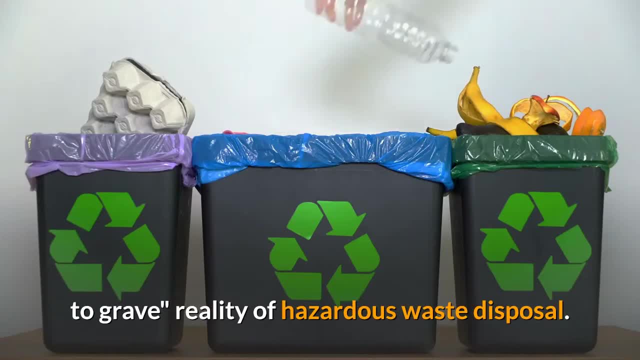 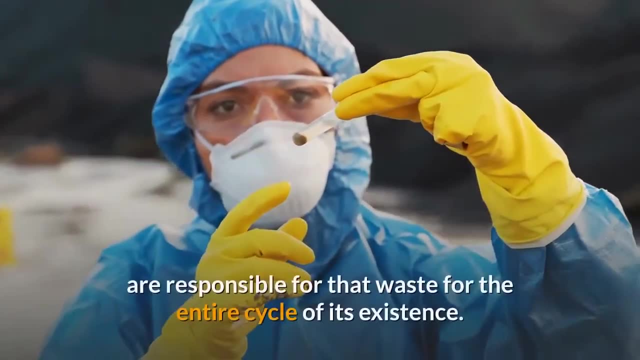 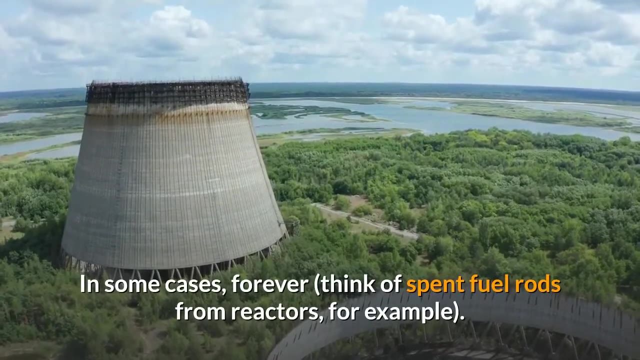 Let's take a short trip down the Cradle to Grave reality of hazardous waste disposal. Cradle to Grave Hazardous waste means that you, as the generator of hazardous waste, are responsible for that waste for the entire cycle of its existence, In some cases forever. think of spent fuel rods from reactors, for example. 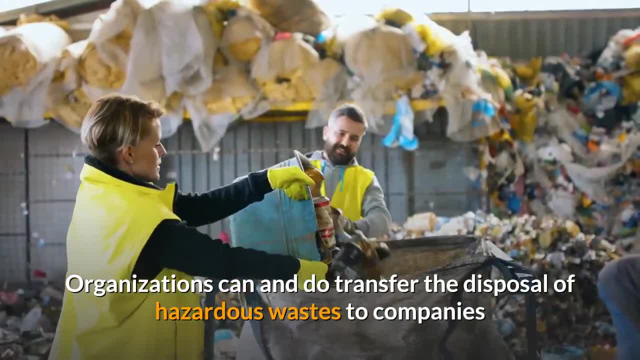 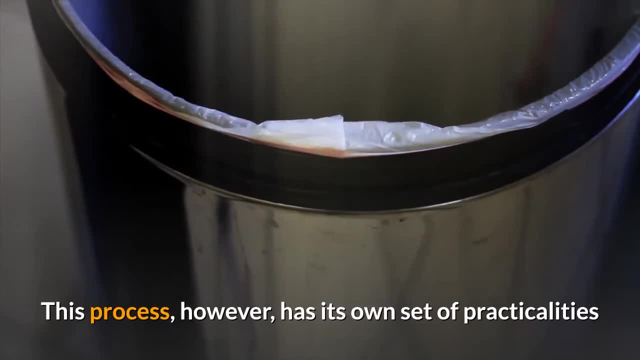 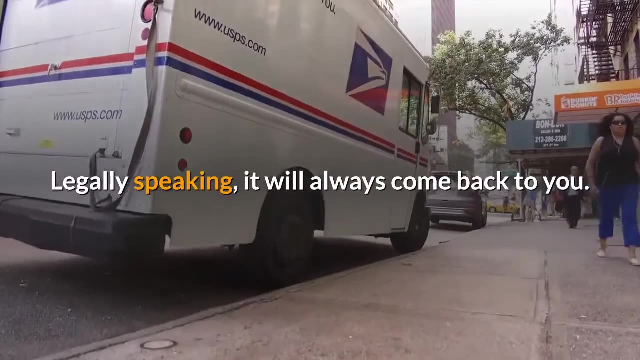 Organizations can and do transfer the disposal of hazardous wastes to companies that are in that business. This process, however, has its own set of practicalities that require you to be very careful when selecting who handles the disposal for you. Legally speaking, it will always come back to you. 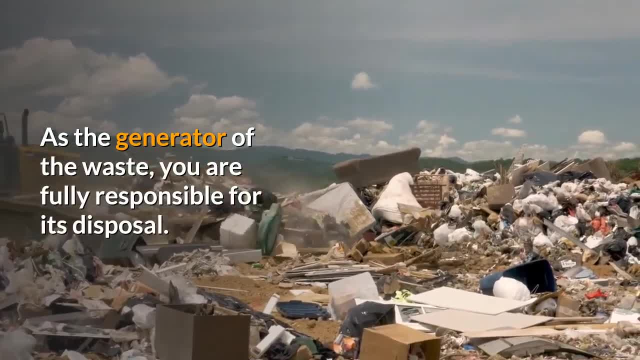 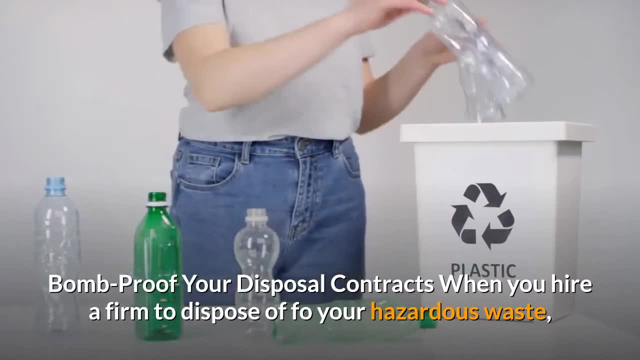 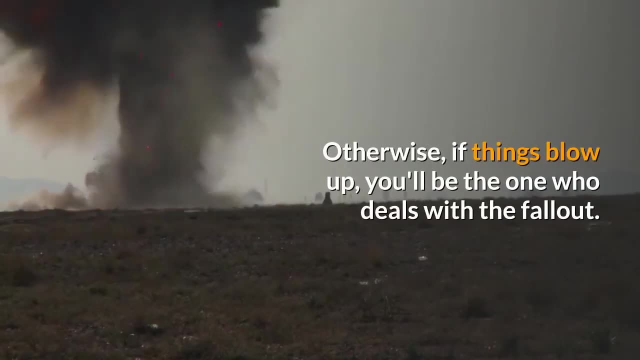 As the generator of the waste, you are fully responsible for its disposal. Bomb-proof your disposal contracts. When you hire a firm to dispose of faux-year hazardous waste, make sure the contract you sign with them is bomb-proof. Otherwise, if things blow up, you'll be the one who deals with the fallout. 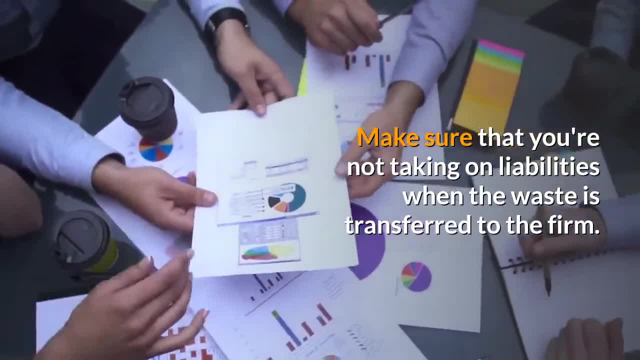 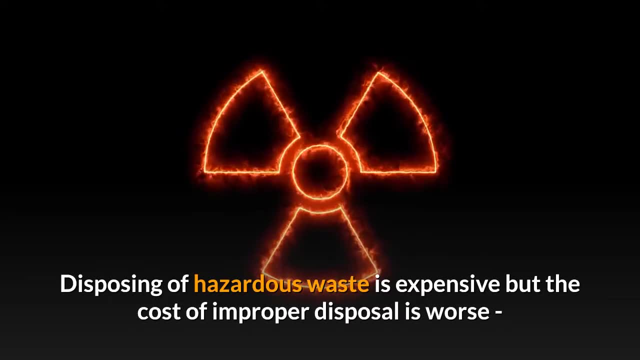 Make sure that you're not taking on liabilities when the waste is transferred to the firm. Disposing of hazardous waste as a result of hazardous waste disposal. Disposing of hazardous waste as a result of hazardous waste disposal. One of the most important tips is that a hazardous waste disposal vacation is expensive, but the cost of improper disposal is worse. 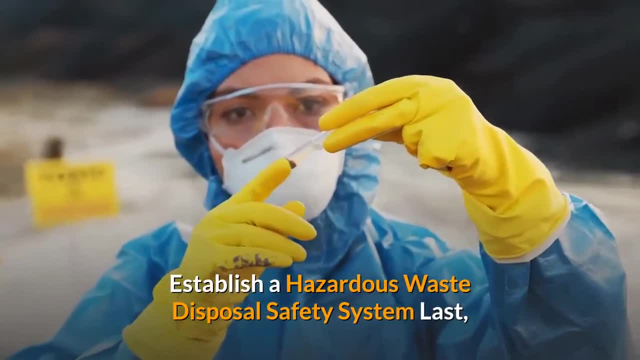 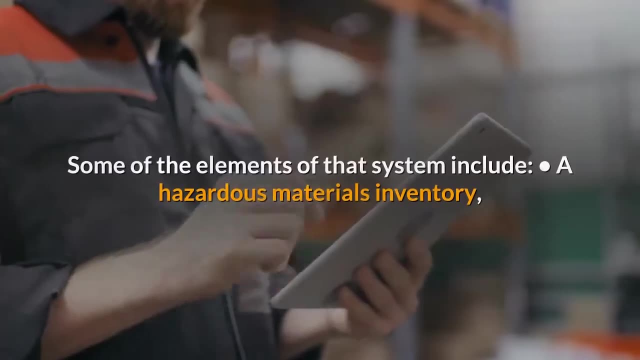 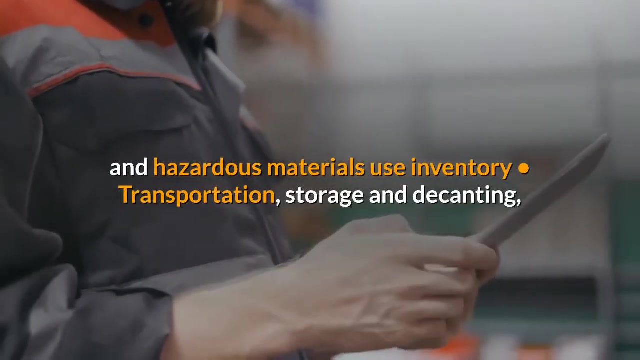 Also make sure the contract language is clear and airtight. Establish a hazardous waste disposal safety system. Last, the disposal of hazardous waste requires a safety system. Some of the elements of that system include a hazardous materials inventory and hazardous materials use inventory, transportation, storage and decanting, labeling, response, exposure and spill control.